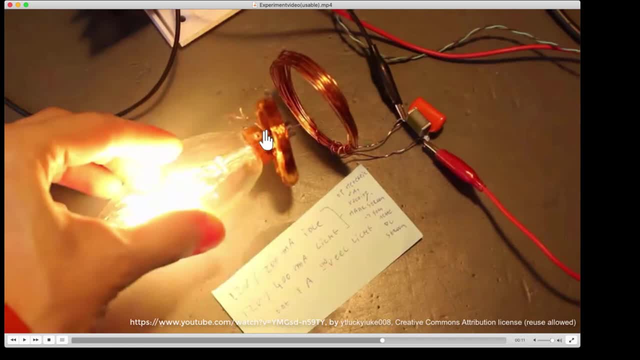 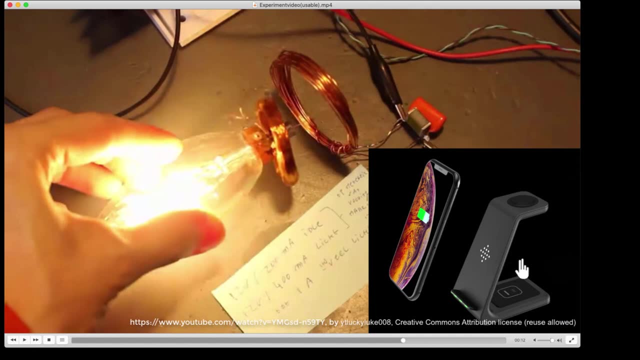 a wireless power transfer. electricity transfer from one coil to another. There is no connection between them, And the idea is the same in wireless charging phones. There is a wireless power transfer happening, So how is the electricity able to jump from one wire and enter into? 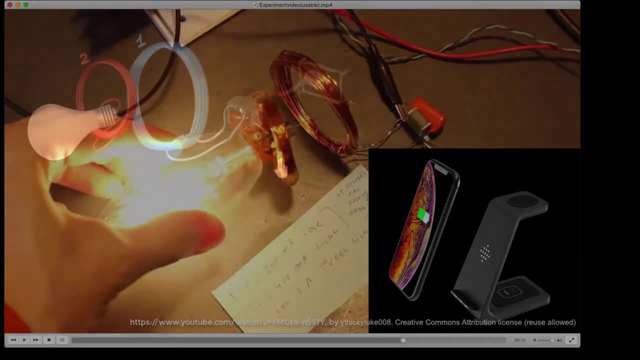 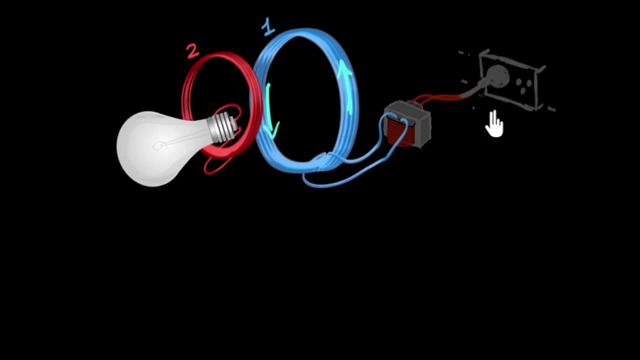 another wire when there is no contact, Let's find out. So here is the same setup. There is a current that is running through one of the coils. Let's call that as coil 1.. And let's call that current I1.. And everything related to this coil. let's keep it blue. 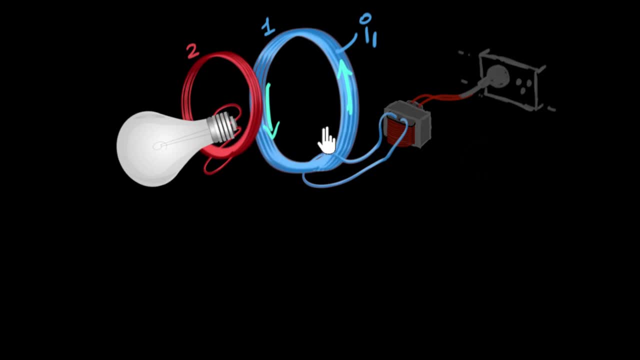 so that we can differentiate between the two coils. And so, because of this, somehow the bulb is lighting up in the second coil. How is that happening? So let's think about this. We know now that the current in the first coil generates a magnetic field in the first. 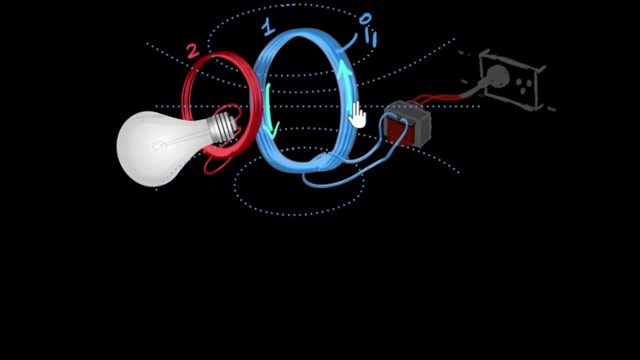 coil. But what's important is that this current is changing. It's continuously changing its direction. Its strength is changing, Which means that the magnetic field that it's producing is also changing. It's fluctuating, And we know from Faraday's law that a changing 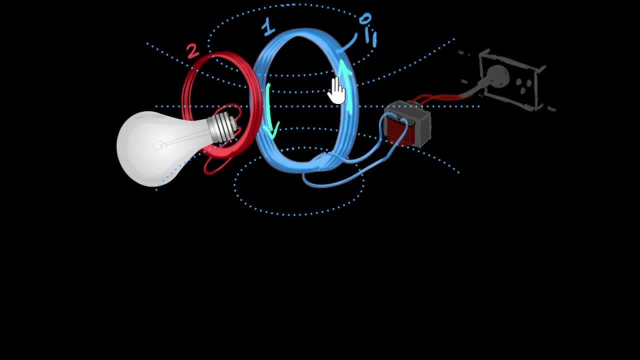 magnetic flux induces an EMF. And so what's going to happen? there are a couple of things that are going to happen. One thing that's going to happen is that this coil itself will oppose the change in the flux, And therefore we say that the coil itself opposes the change. 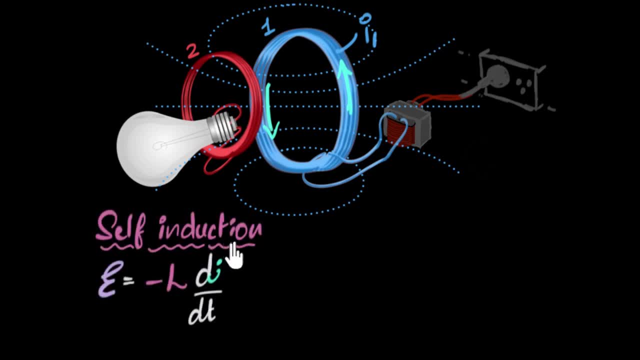 in its own current. This idea is what we call self-induction, Because the opposition is happening to the same coil. So there's an EMF induced in this coil And so what's going to happen to this coil due to the change in its own current Self-induction. However, 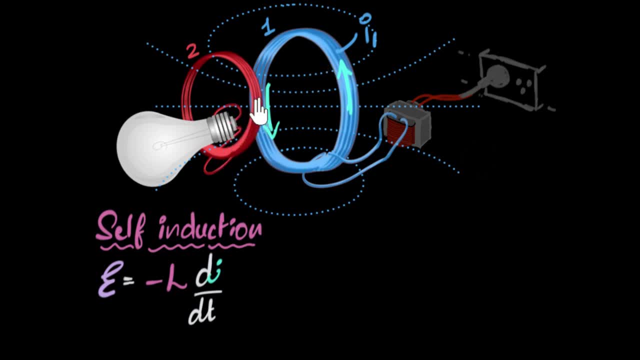 this time. what's happening in this experiment is that this field, generated by the first coil, is also seen by the second coil. It's also linked with the second coil, as you can see, And therefore, if the field is changing, the flux through the second coil is also changing. 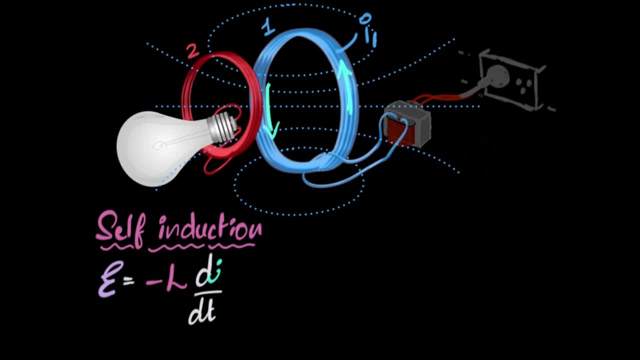 This means there will be an EMF induced in the second coil as well. So let's write that There will be an EMF induced in the second coil. Due to what? Due to changing current in the first coil. This idea where you have an EMF induced in one 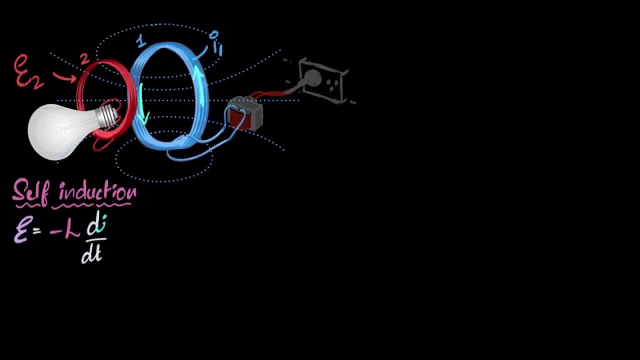 coil due to the changing current in the another coil. That's what we call mutual induction, And we'll get to know exactly why it's called mutual in a second. But that's the idea behind mutual induction. Hopefully you can differentiate between the two now. 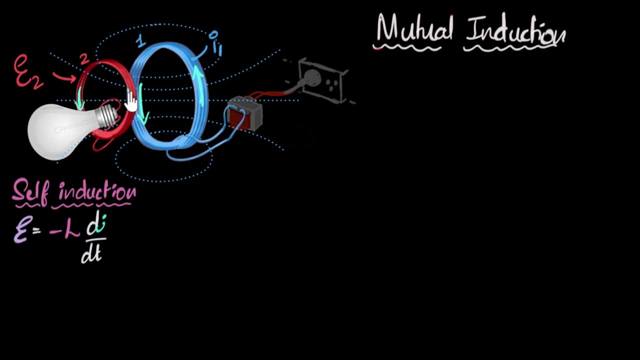 And because there's an EMF induced over here, there's a current that starts running over here and that induced current causes the bulb to glow, And that's what we saw in our experiment. Pretty cool, huh. That's how wireless power transfer works. But we also saw that when 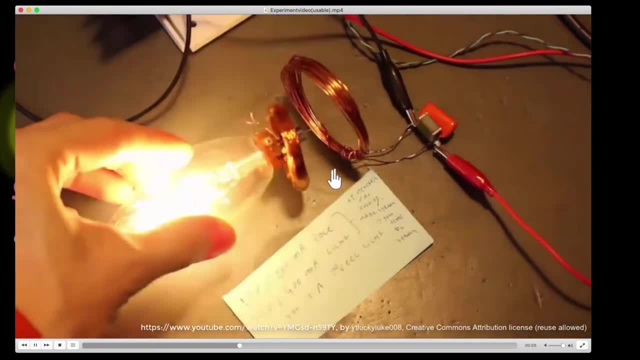 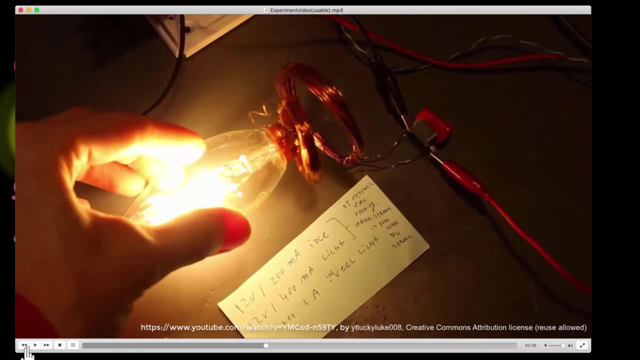 you take that. when you took that secondary coil far away, notice the bulb stopped glowing. It's only when you come closer it glows. Why did it stop glowing if you took it far away? Can you now answer this question? Well, when you take it far away, the magnetic, the strength, 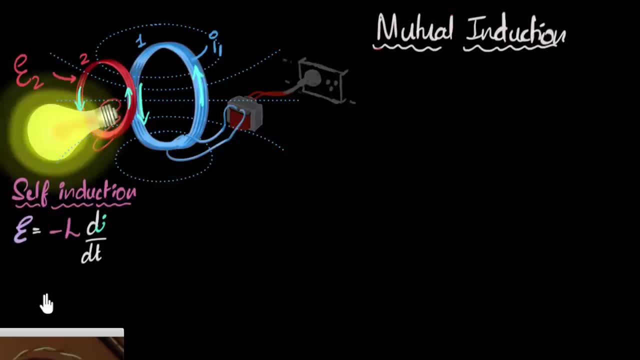 of the field reaching this coil becomes very weak. In our diagram you can see that if you now take this far away, the magnetic field linked with this coil becomes very weak And so the flux changes are very weak. Induced EMF is very weak And, as a result, the current 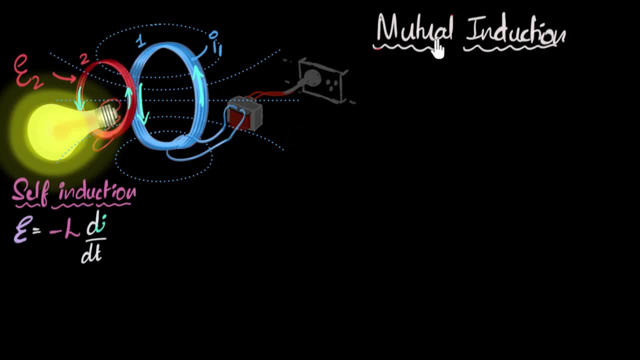 induced will be smaller and the bulb won't glow. Okay, now let's go ahead and write an equation for mutual induction, And I want you to take a shot at it. It's going to be very similar to this equation, but this is the self induction happening in the same coil. 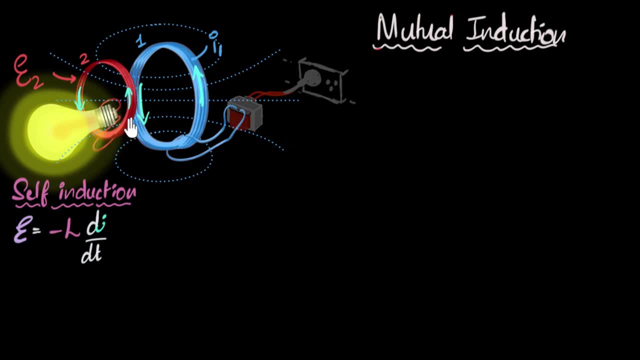 Let's take a shot at it. Okay, so here we just have to be careful about which coil you're talking about, which currents and which EMFs we're talking about. So we're talking about the EMF in the second coil. So EMF, E2 equals minus. here we had self inductance as the constant. 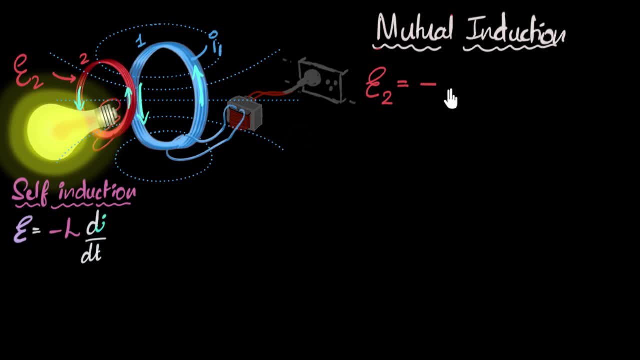 here we'll introduce a new constant called mutual inductance and we'll talk a little bit about it. But who is mutual inductance? Is it the second coils or the first coils? The second coils, right, Because induction is happening in the second coil, So minus. 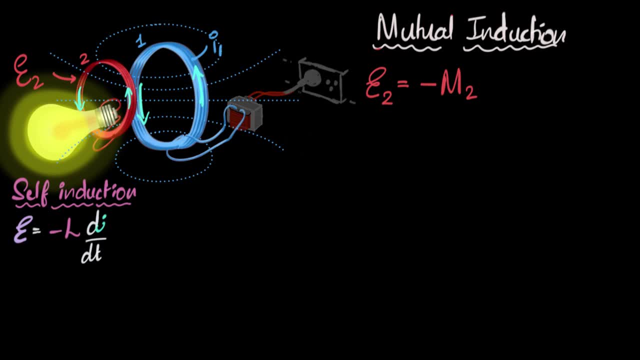 M2, I'll write times DI over DT. but which DI over DT? Is it the rate of change of the current of the second coil or of the first coil? Hey, it's of the first coil. That's the whole idea behind mutual induction. EMF is induced in the second coil due to the current. 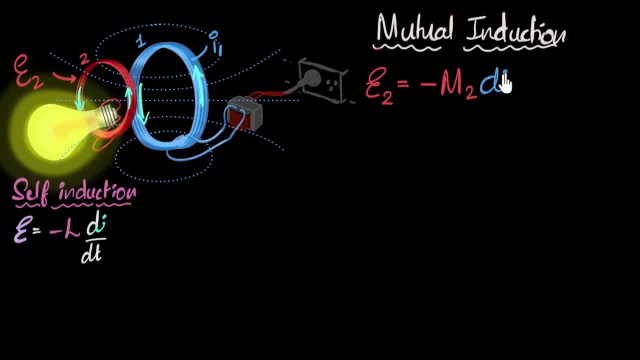 changing in the first coil. So we'll write DI1 over DT. And this mutual inductance, just like self inductance, has units of Henry And if the value is very high it means that a EMF is induced when the current changes in the other coil. And what does its value depend? 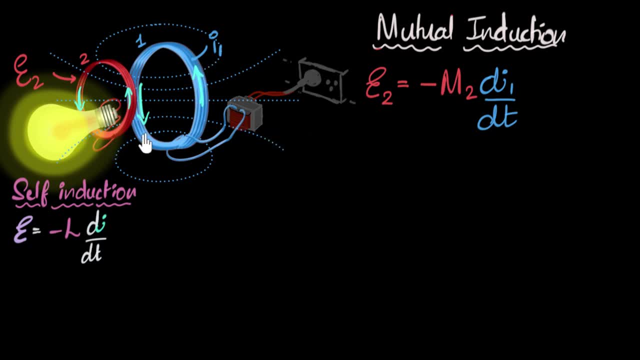 on. Well, just like self inductance, it does not depend on the voltages or the currents. It's a matter of geometry. It depends upon how many turns this coil has. what's the radius of this coil? It also depends upon how far it is from this coil. The farther you go. 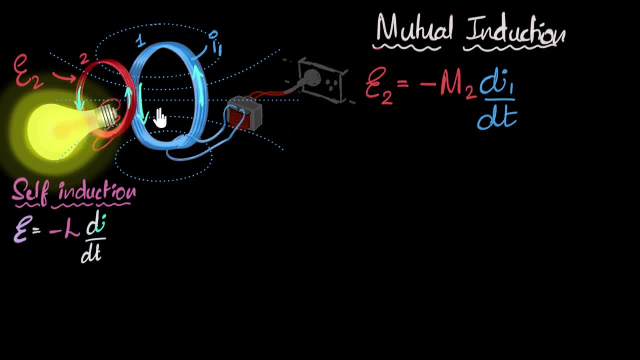 the mutual inductance drops. The closer you are, the stronger the mutual inductance, The orientation, how they are kept together. It also depends upon the number of turns of the first coil. That's right. It depends on that as well, And we will calculate mutual inductances for. 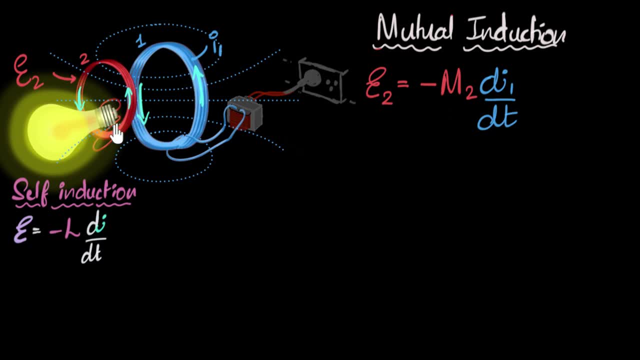 some cases in future videos. But since the mutual inductance of the secondary also depends upon the properties of the primary, we like to often say that this is mutual inductance of the second coil with the respect to the first coil, And this will make sense if you. 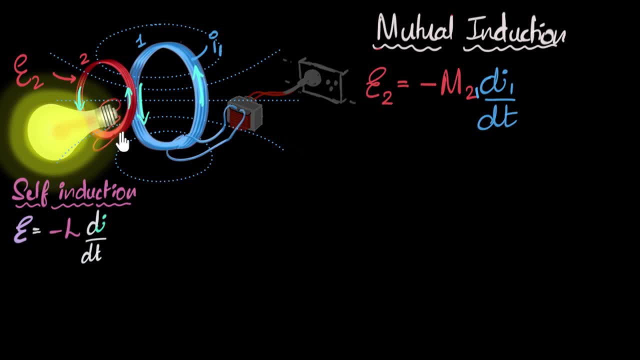 think there are many other coils in world over here. then there will be a mutual inductance between two one, mutual inductance between two- three, mutual inductance between two- four. So for every pair of coil there'll be a value for mutual inductance, And that's why we like 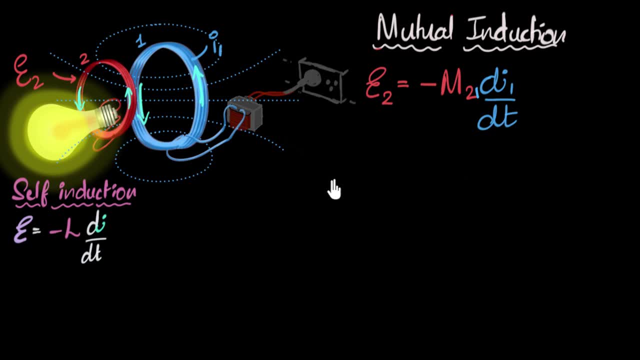 to write two one over here. Okay, Now, here's where things get really interesting. So because of the EMF generated in the secondary coil, there is a current induced. in the secondary coil right, There's a current induced, and that's then. that's why the bulb is glowing. 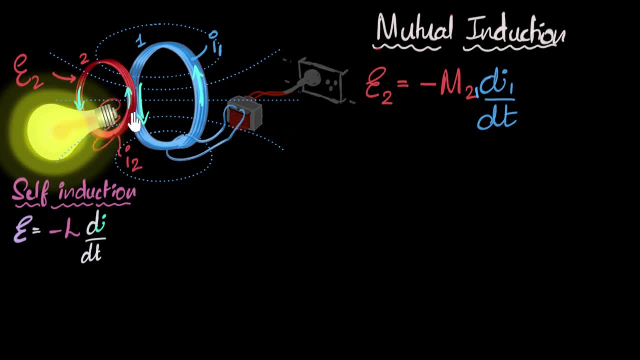 But now think about this: This current also generates its own magnetic field. So here is the magnetic field, The magnetic field generated by this current, And because this current is also changing, this magnetic field is also changing And as a result of that, it induces an EMF in. 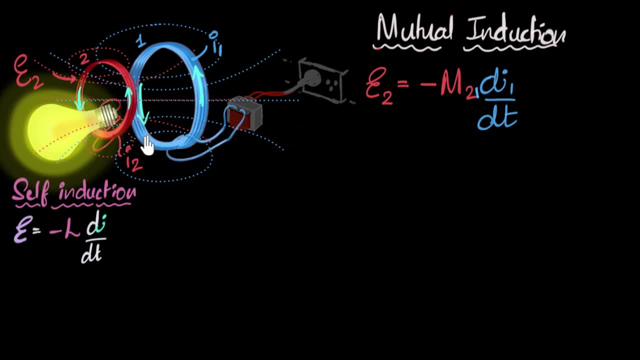 the primary And therefore, because of the changing current in the secondary, there will be an EMF induced in the primary as well And we'll have a very similar formula. And I want you to, you know, take a shot at writing this down. but now, hopefully you understand. 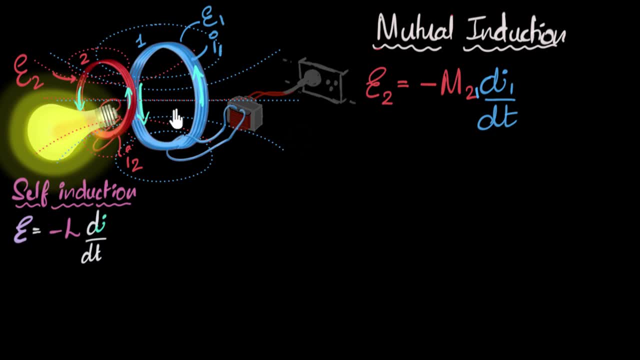 why it's called mutual inductance? Because they both induce EMF in each other. That's why it's called mutual induction. So can you now pause the video and write down what would be the expression for the EMF induced in the primary coil? 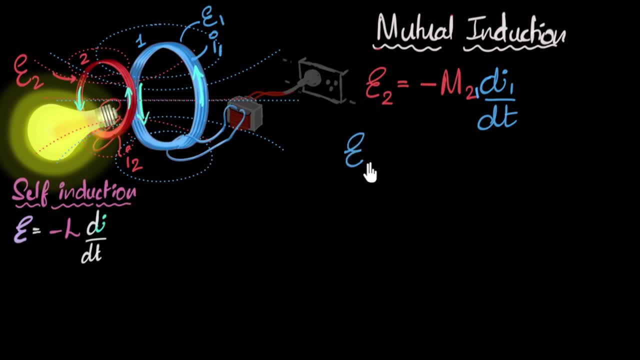 All right, So we're very similar. It's going to be: EMF induced in the primary coil is going to be negative. mutual inductance of the primary coil times the rate of change of current of the secondary coil. Remember it's always the change in current of the other coil. So 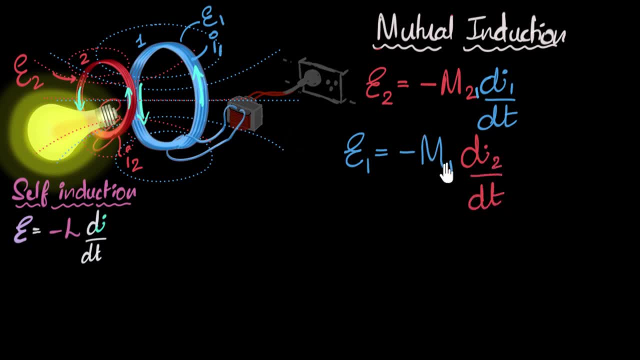 it's the change of current of the other coil And, again for similar reasons, we will write this as mutual inductance of the primary with respect to secondary, And the same thing holds over here. This is also, Henry. This also depends upon the configuration, geometry and all of 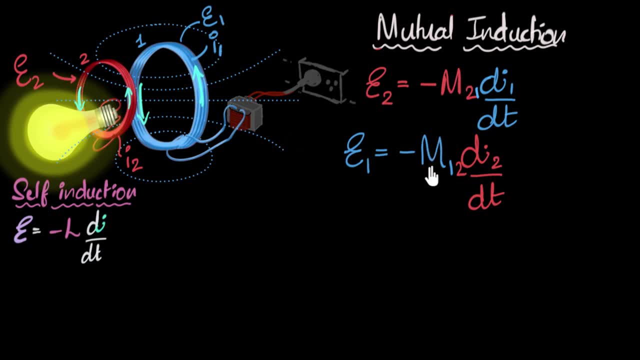 that. And finally, there is a very nice, surprising connection between the two mutual inductances. See, when I was learning this, if you were to come to me and ask, Hey, what is the relationship between M12 and M21? I would say I have no idea what the relationship would be right. 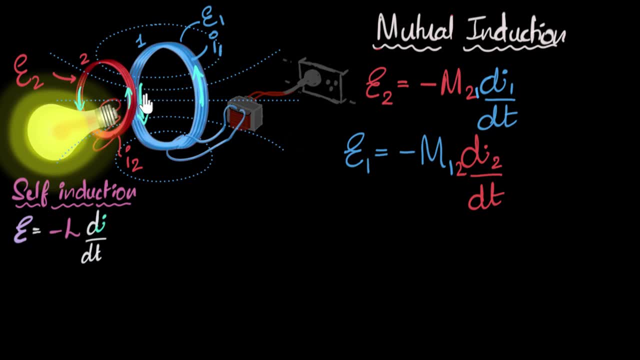 why should there even be a connection between the two, right? well, however, it turns out that those two values will always be equal to each other, and that's right. you have to box it with the exclamation mark, because this is by no means obvious, but that's great, it makes our lives easy. 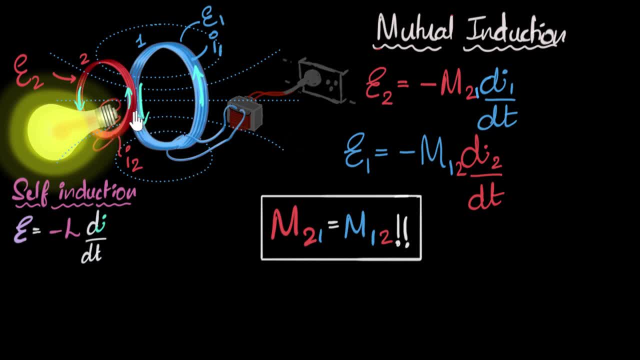 so what this means is, if you have a pair of coils, then there is one single value for mutual inductance. whether you consider its mutual inductance of this coil with respect to this, or you consider this coil with respect to this, turns out to be the same, and this is super useful. 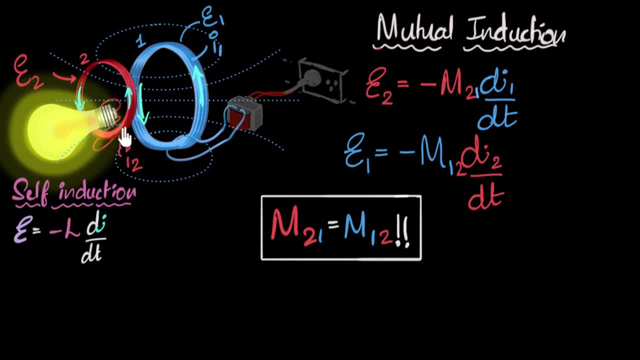 when you're calculating mutual inductances, because you can decide which one you want to calculate and sometimes, and in fact most times, one of them is always easier to calculate. another one is almost impossible, and we'll explore all of that in future videos. and one final thing for folks who 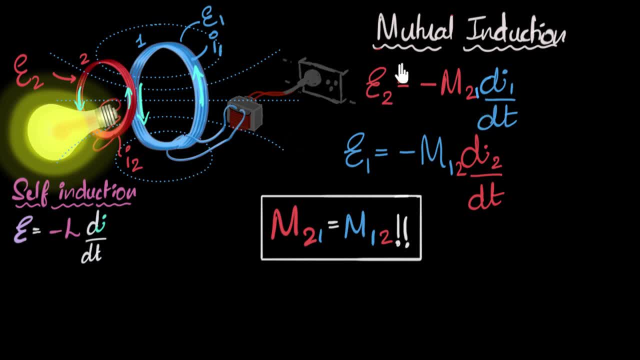 are really curious. these are not complete equations because this emf is only due to mutual induction. remember, there will be an emf induced due to its own changes in the current, so the complete equation would be a mutual induction. along with that, there will also be self-induction, which is caused due to changes in its own current.